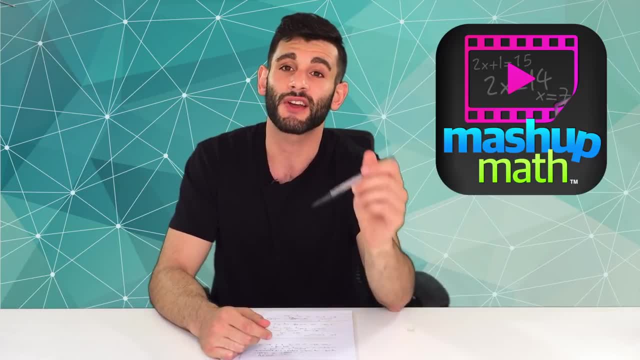 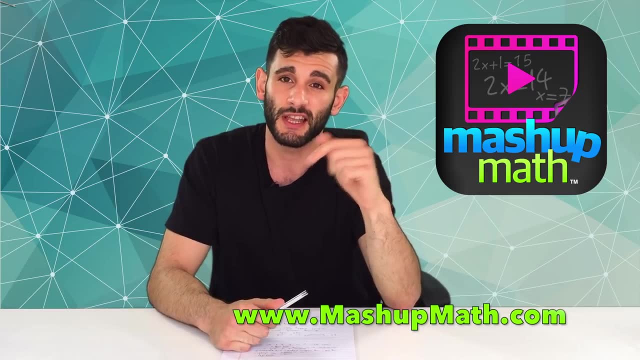 things for yourself. Now, if you want a little bit more structure, there is a free worksheet available at mashupmathcom in our resources section, And that link for that worksheet is in the description below. So just go ahead right there and grab that before you start, If you want. you do not need it. You will need the materials that. 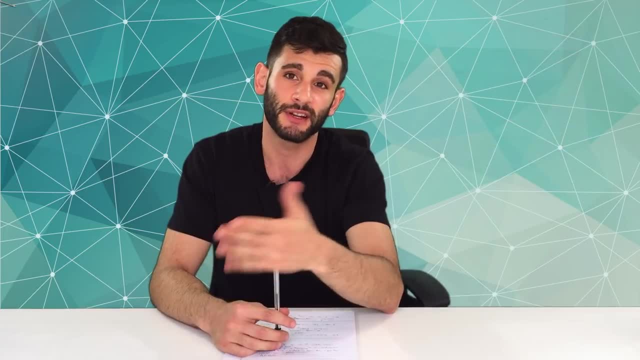 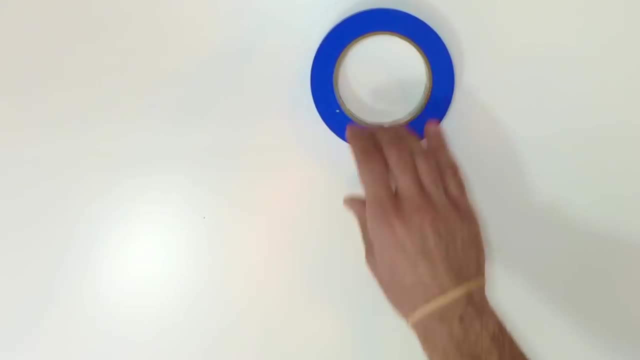 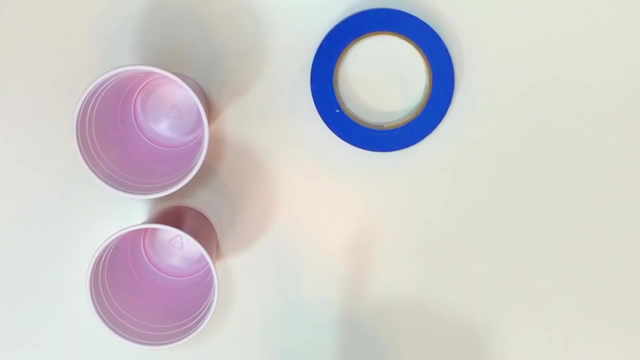 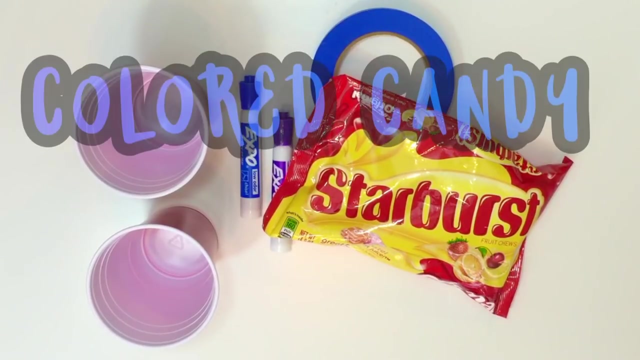 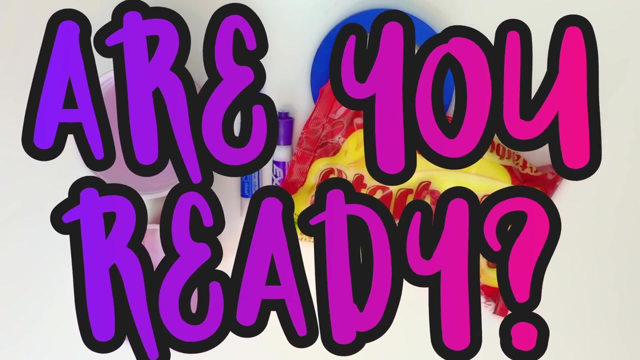 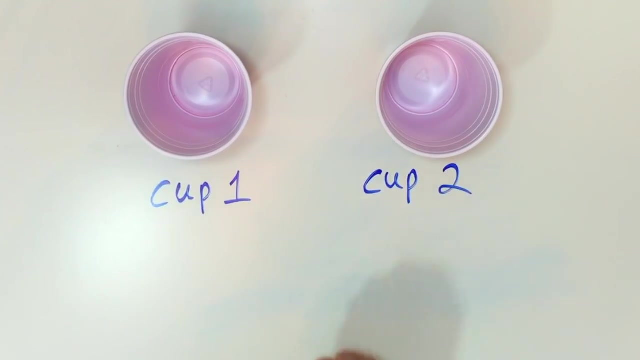 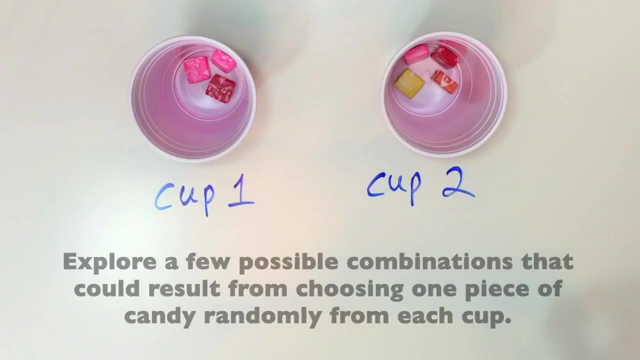 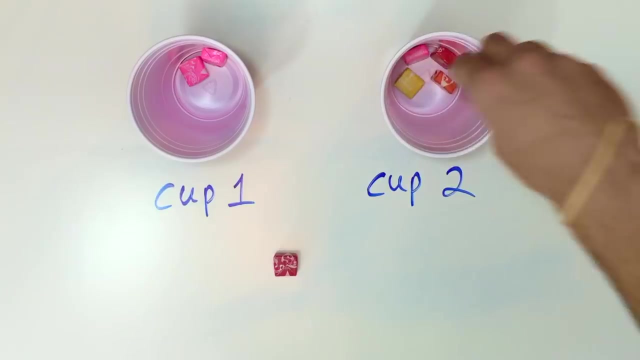 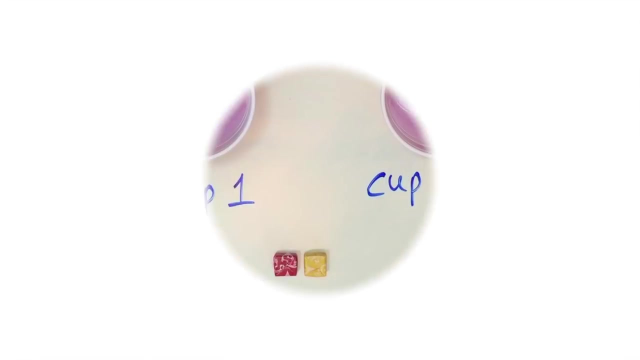 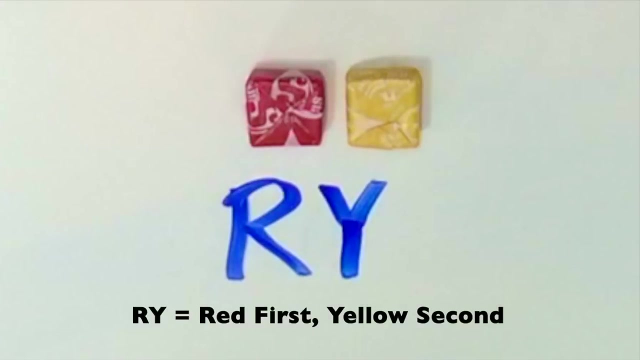 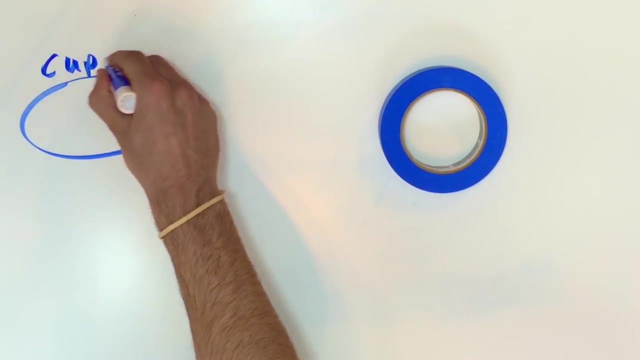 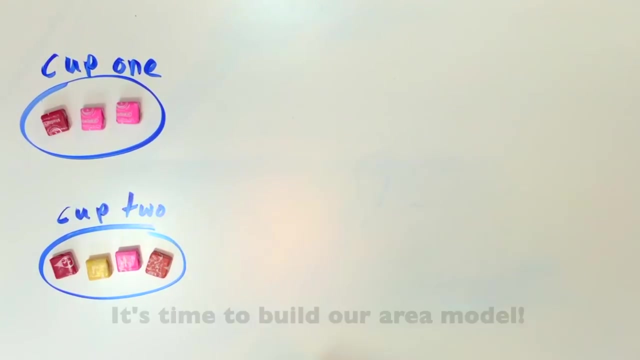 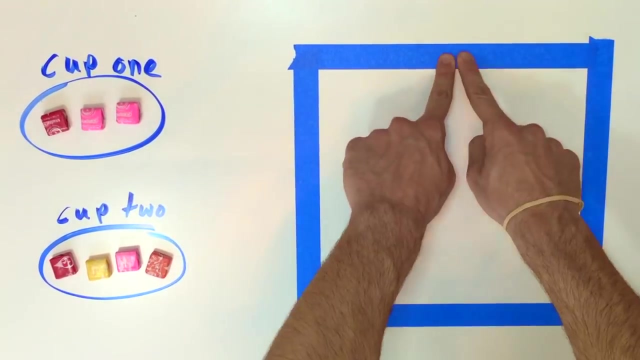 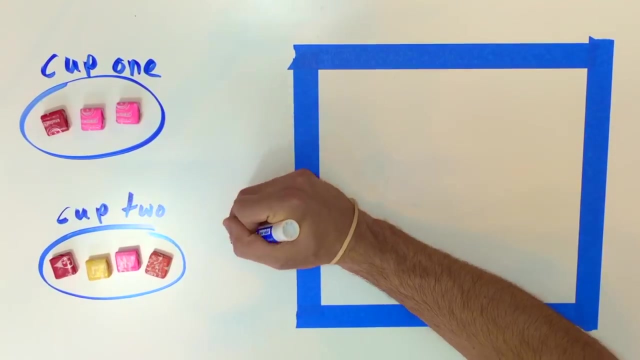 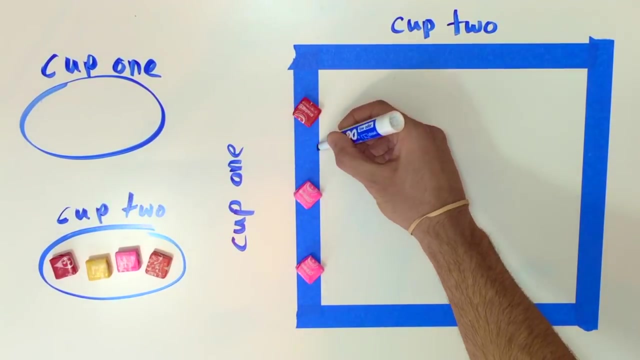 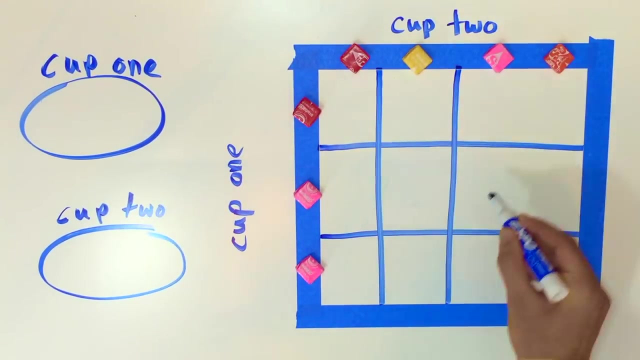 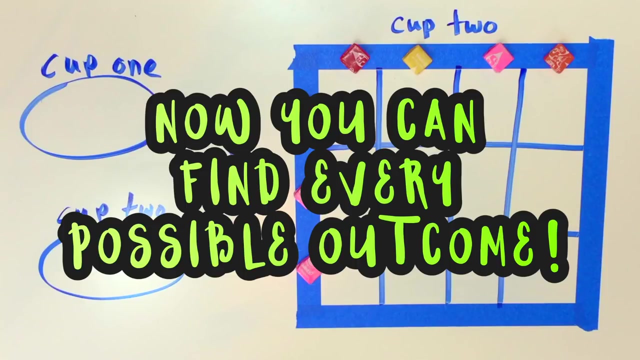 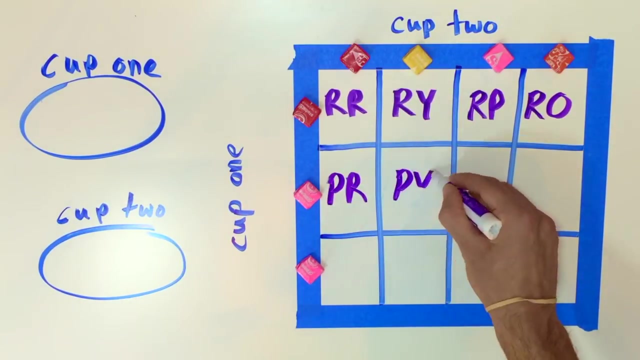 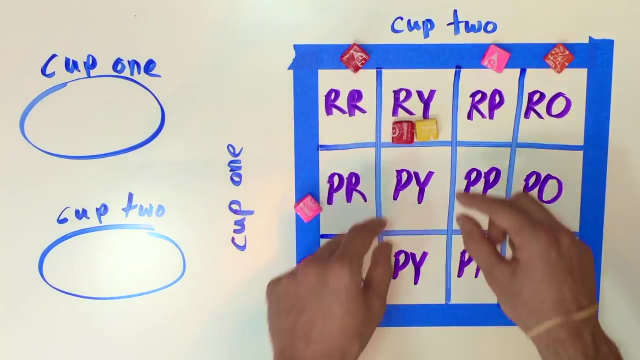 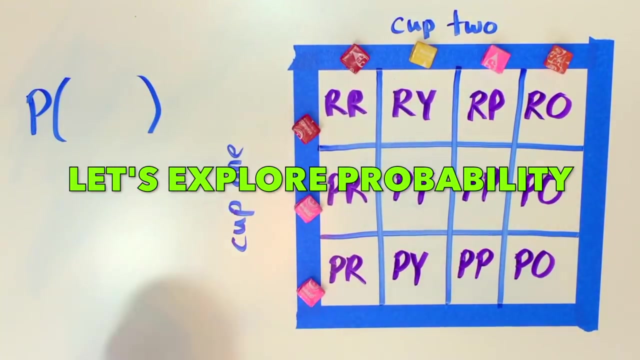 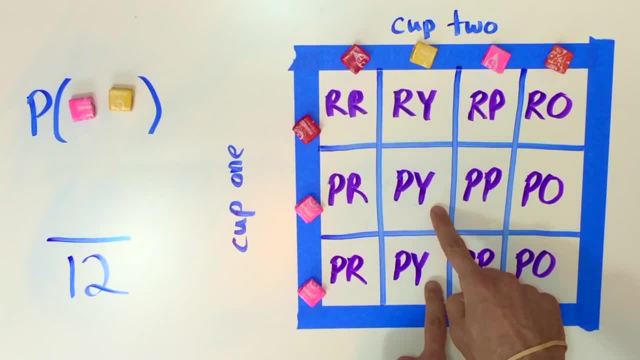 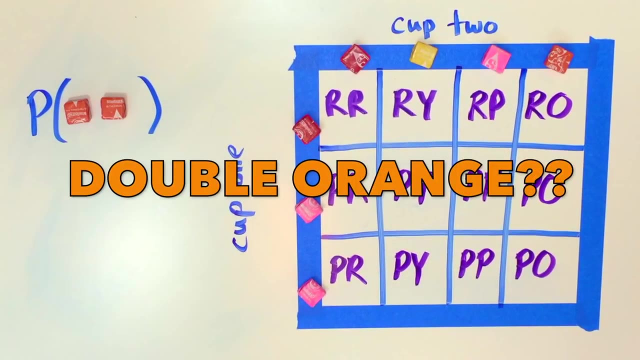 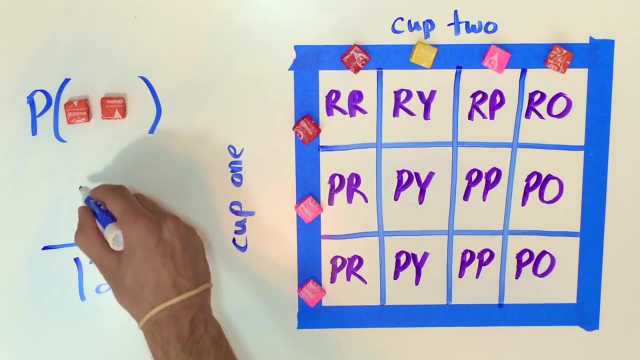 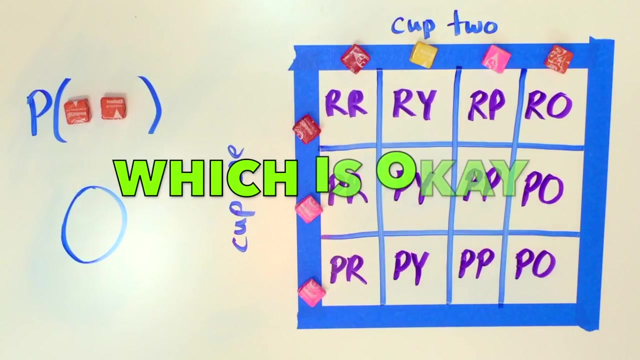 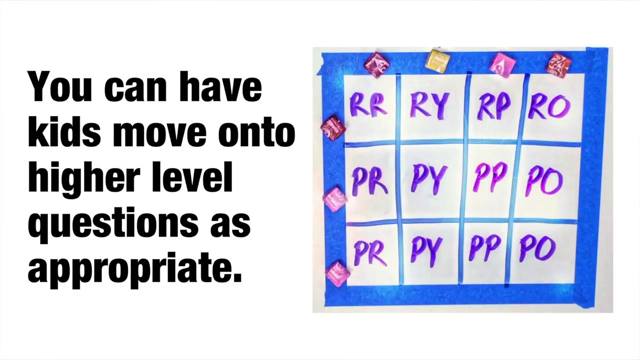 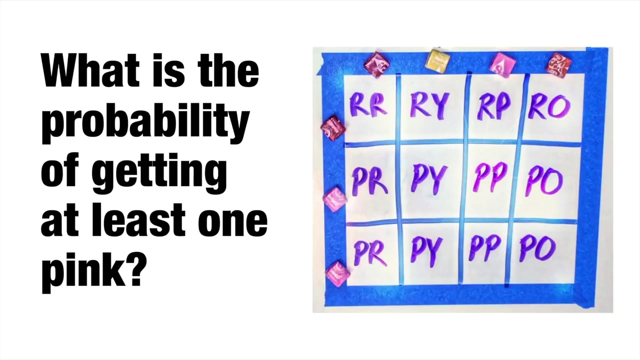 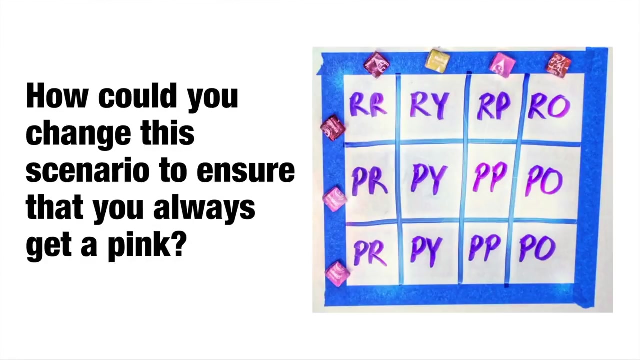 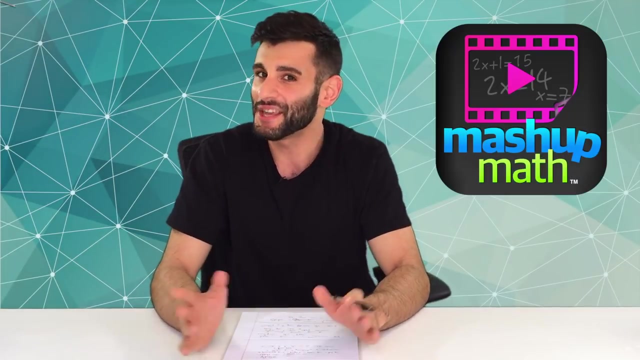 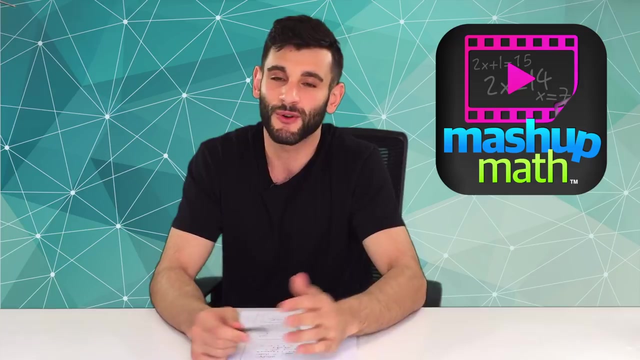 Thank you. Thank you, All right, so that's the activity I use, Starbird First. you can use any kind of candy you want, as long as there's some variety with the colors. But be creative, be resourceful. maybe something from a dollar store, whatever works. 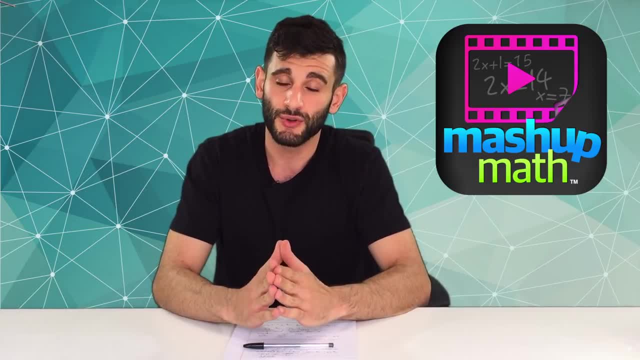 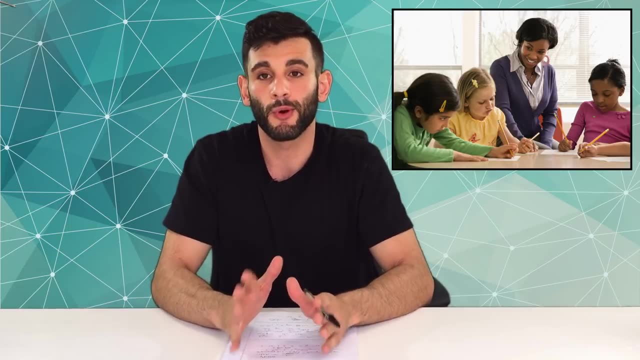 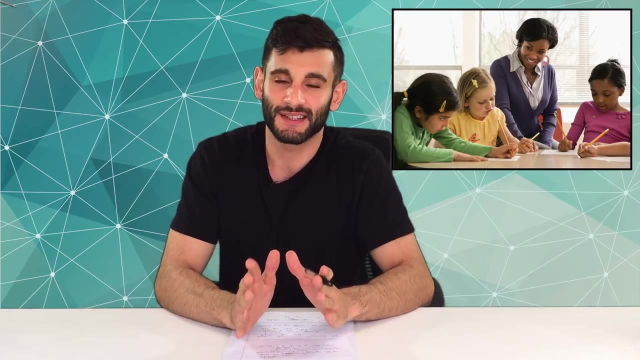 The important thing is that you have something physical to use to represent the scenario in a more hands-on way. And a final reminder: remember: let your students explore, Let them make mistakes, Hold back as much as you can. Only apply structure when you think it's absolutely necessary. 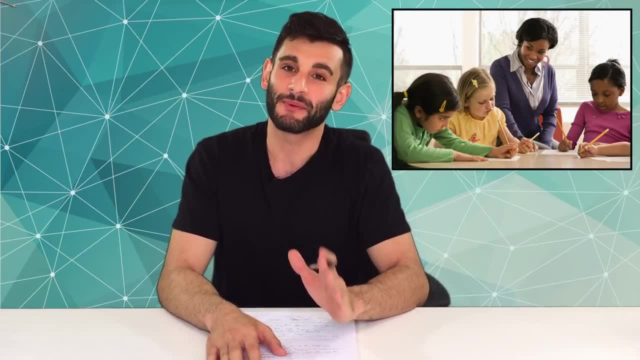 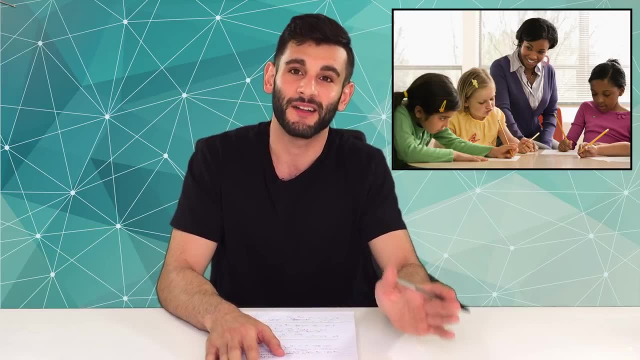 But try to hold back. I know it's hard. I know you want to jump in when you see students making mistakes or when it looks like their thinking is not quite correct, But even if they veer off the path for a little while. 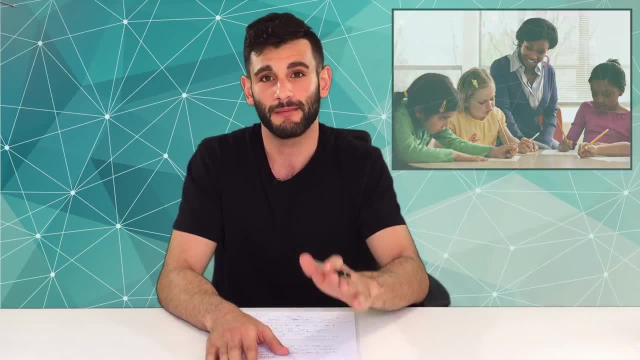 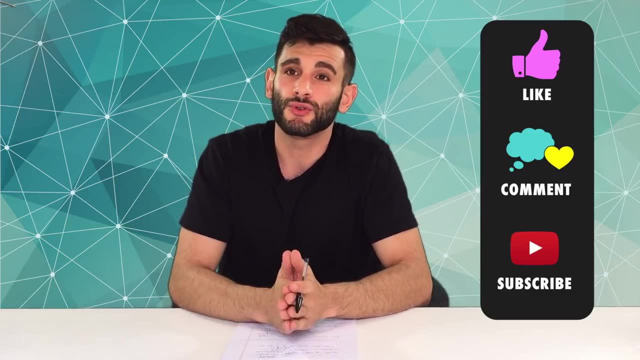 they'll find their way back most of the time, if you allow them to Just keep that in mind. And finally, if you want to support our channel, we have a very simple request for you, And that is to do one of, or all of the following things: 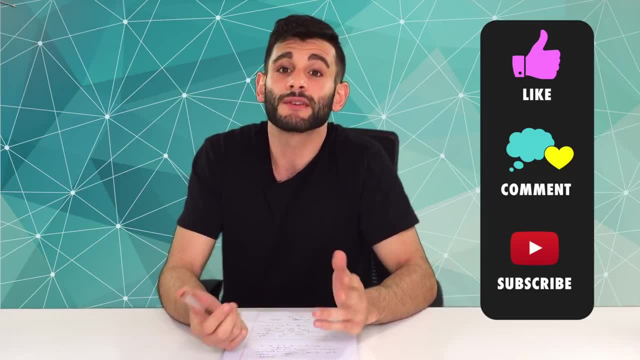 One of those is to hit that thumbs up button and like our video. Number two is to leave a comment. That's the most important one. We want to hear what you're thinking. Comments mean a lot to us. help us to kind of. 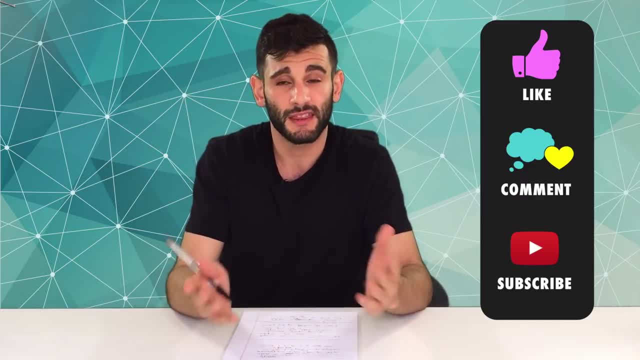 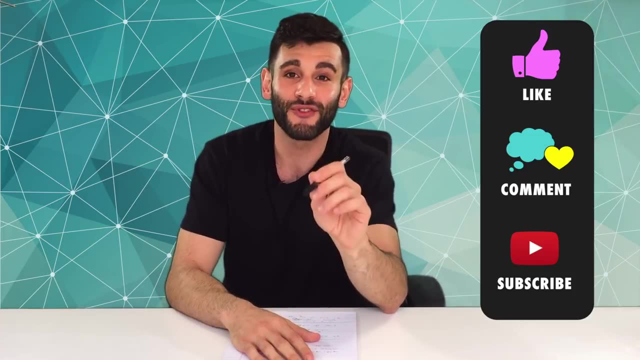 guide what we're going to do next, what our next vlog posts will be, and things like that. So please leave a comment. That would be awesome. Third thing you can do is subscribe to this channel if you have not already. And number four is to share this video. 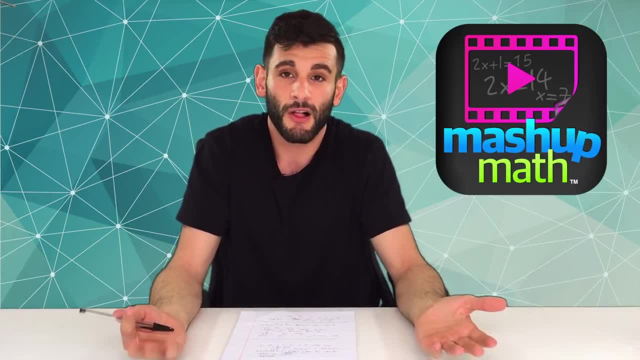 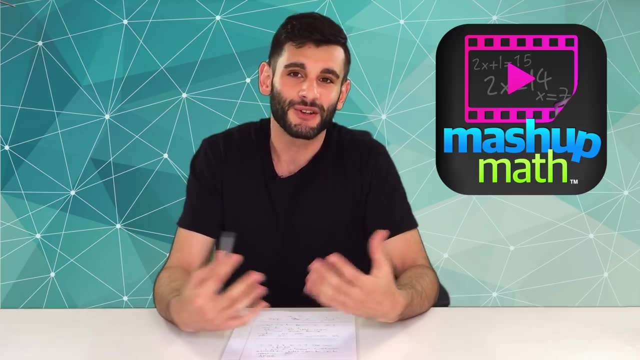 on whatever social media platform you use the most, or all of them. So Pinterest, Facebook, Twitter, Instagram, wherever you are on social media, if you could share our videos, our posts, it would mean a lot, help us to broaden our audience.